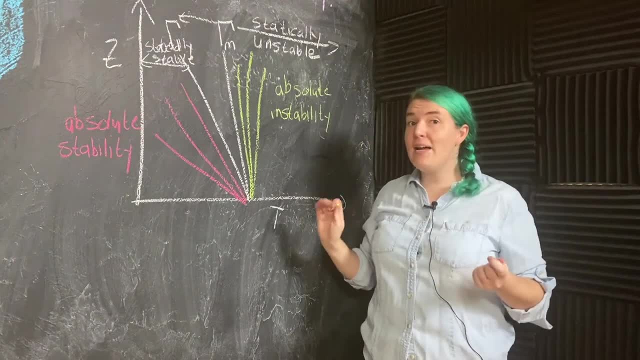 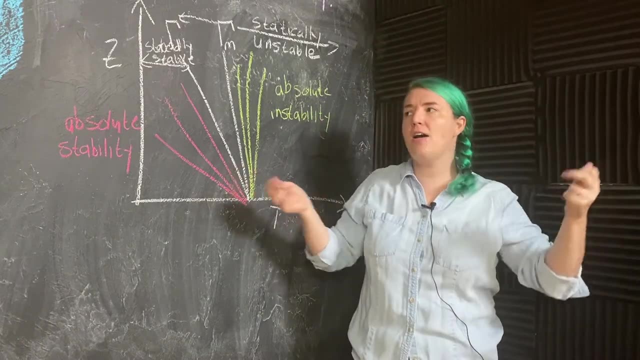 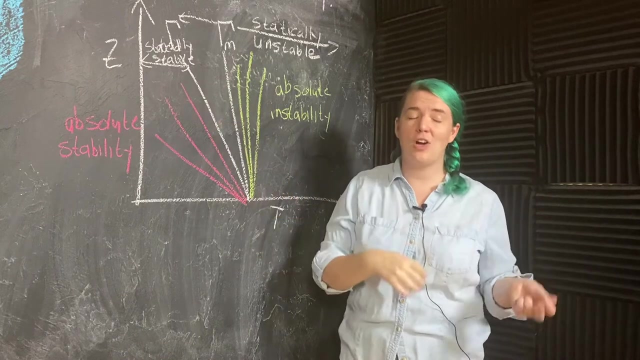 Or absolute instability If my atmosphere is over in this regime. we've got air parcels rising left, right and center, Cats and dogs befriending each other. It's just chaos. But what about this region in between the dry and moist adiabatic lapse rate? 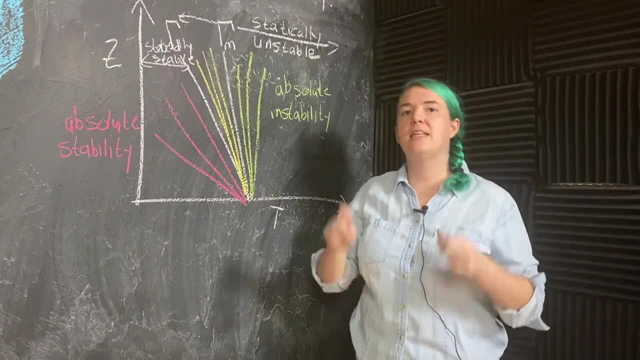 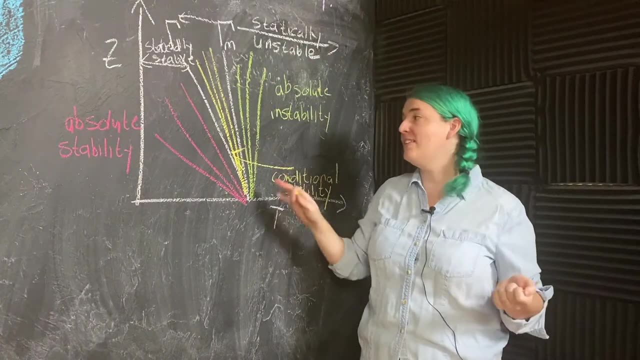 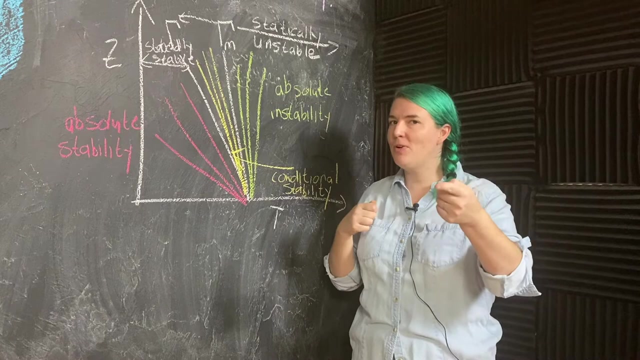 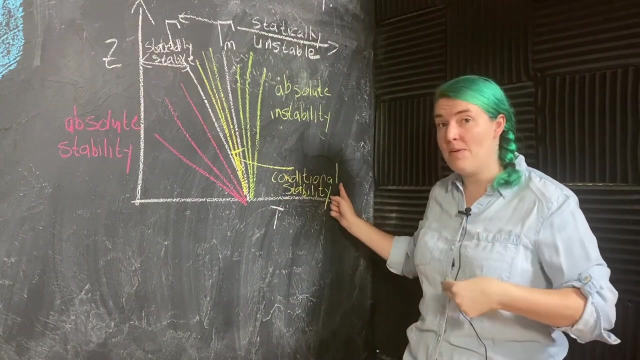 It's in this region I refer to as conditionally unstable or conditional stability. Will an air parcel rise when the lapse rate is in this region? Well, it depends on bonus points. if you guessed this before I say it, Water vapor. If the atmosphere is conditionally stable, then a dry air parcel will be stable. 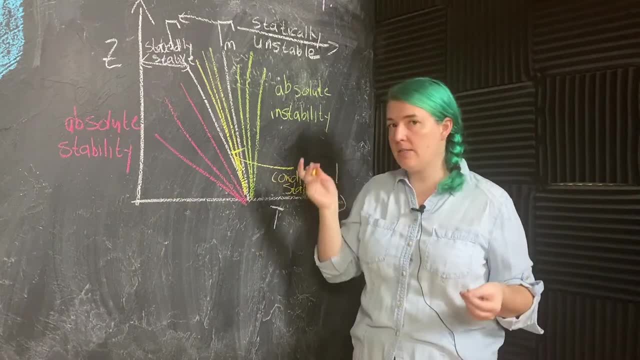 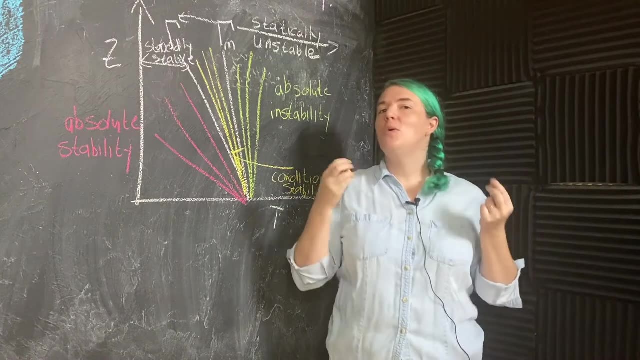 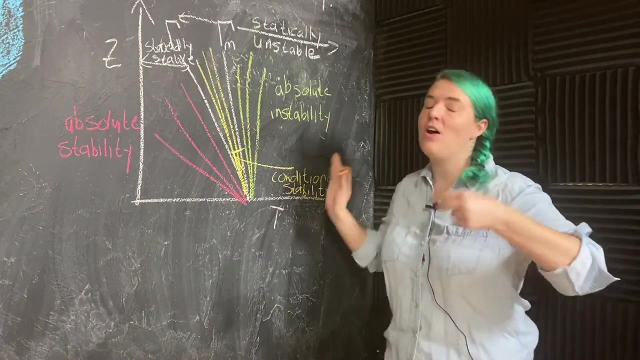 but a saturated air parcel will tend to rise and be unstable. So whether or not an air parcel in this region will rise, whether or not we have a buoyancy-driven lifting mechanism, is conditional on the water vapor that is present that day. That's conditional stability. 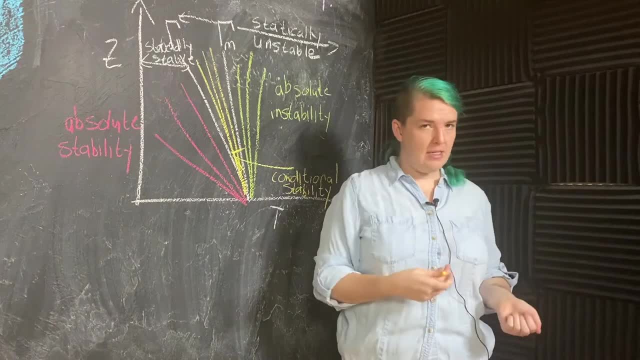 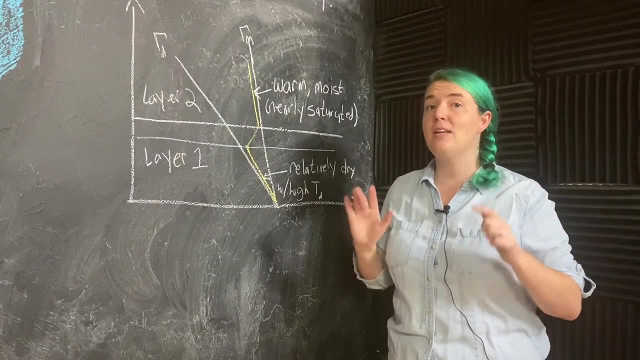 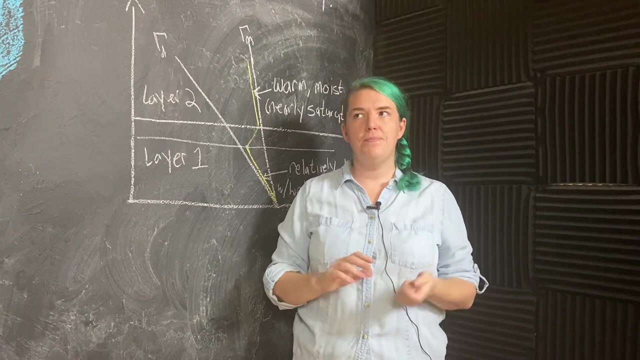 So let's erase this, and now we'll talk about convective stability. In order for the atmosphere to be convectively unstable, we need a pretty specific setup. Before we get into those details, I want you to think about convective instability as like this: 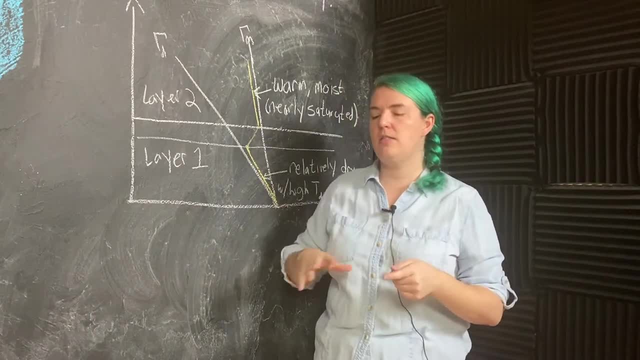 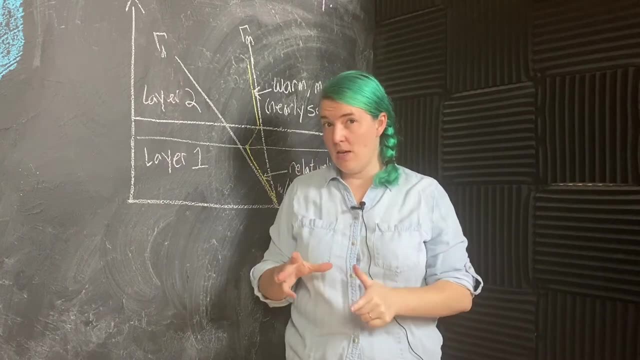 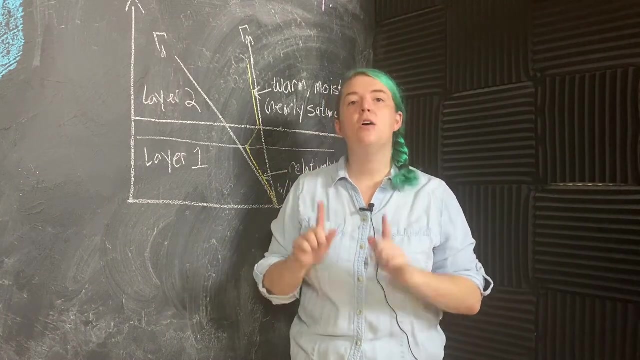 If we have all of the ingredients for a cake and we've made our cake batter and we've put it in the pan, it won't turn into a cake unless someone puts it in the oven. If the atmosphere is convective, then we have all of the right ingredients. 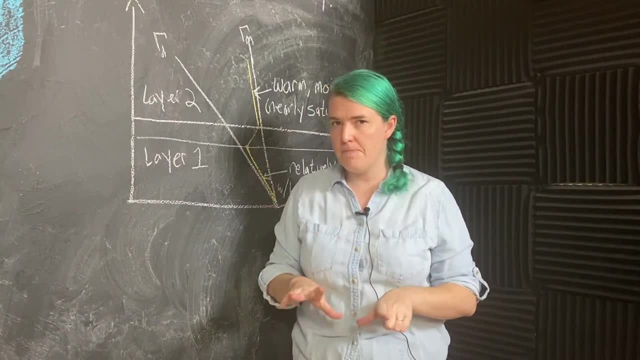 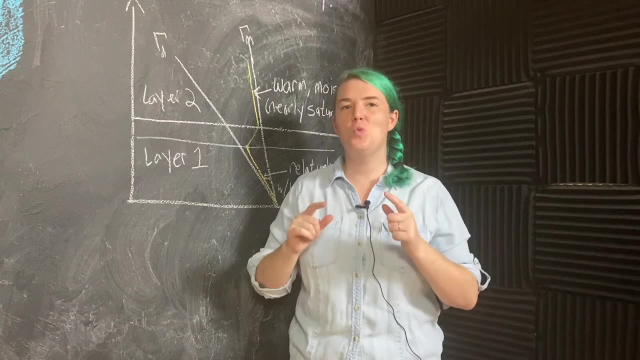 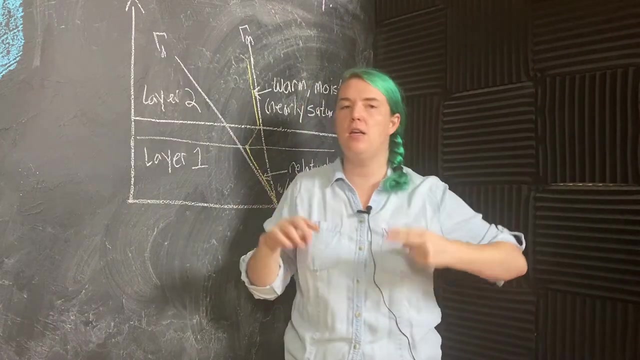 The cake is in that perfect batter state. But to get the actual rising motion, to get that real lifting mechanism, we need something to kick us off. We need to kickstart the motorcycle, We need to put the cake in the oven. Other analogy: 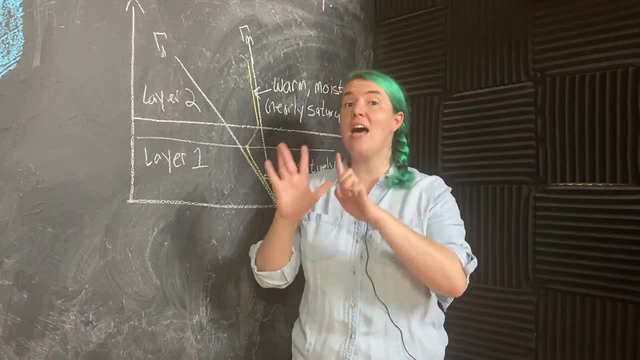 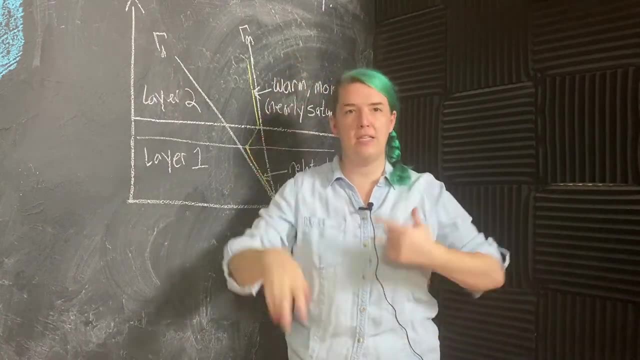 So when the atmosphere is convectively unstable, it is set up so that if something, if something kickstarts it, then we get a lot of convection, We get a lot of rising motion. The setup that we need to have: convective instability.